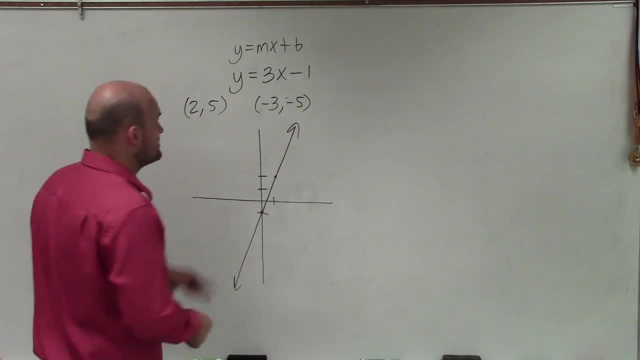 that there's a line, So infinite many points right. So it's possible that both of these points are on the graph. It's also possible that both of these points are not on the graph. OK, So to determine if they are or if they're not, we need to plug them in because they're both coordinate. 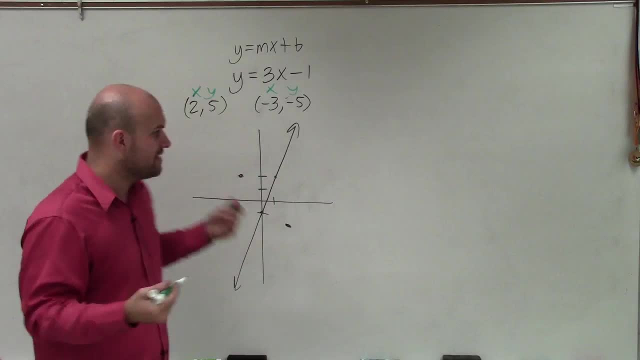 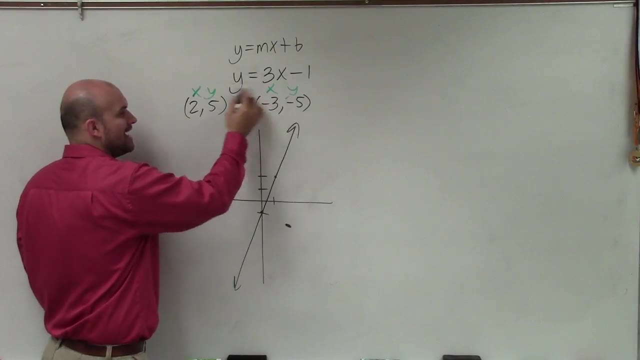 points. That means they both have an x and a y coordinate to them that create the point. So notice how here this is xy, this is xy, And y equals 3x minus 1.. So we're going to plug in a 3u and a 1u of x that are on the ne experiments. So 2x, the integral u, p minus. 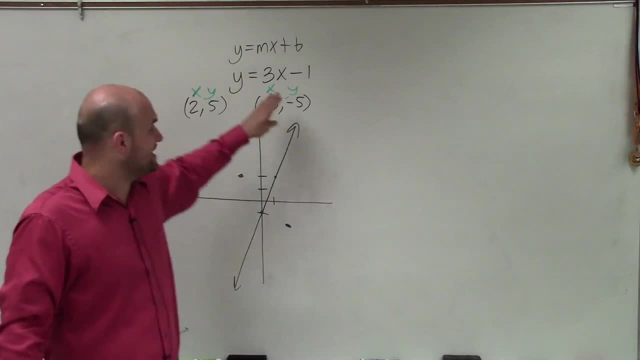 1 represents saying all points that lie on the line are going to make this equation true for any x and y value that are on this graph. So therefore, if I take these points and I plug them into this equation and it makes the equation true, then that point is. 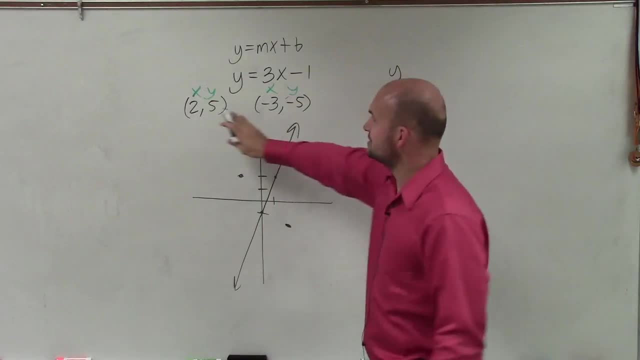 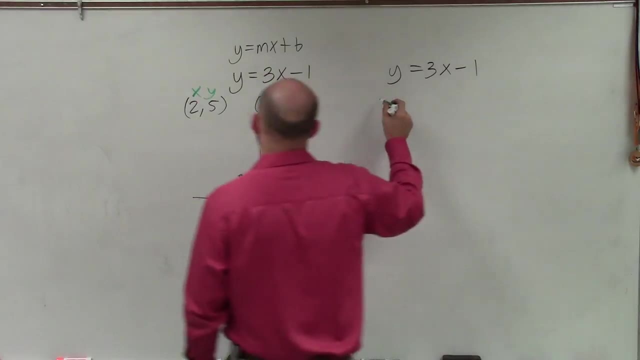 on the line. So let's give it a shot. Let's test our first point: 0,5.. So I have y equals 3x minus 1.. All I'm simply going to do is plug in a 54.. іx- explode. y equals 3x minus1.. All I'm simply going to do is plug in a 54x and a. 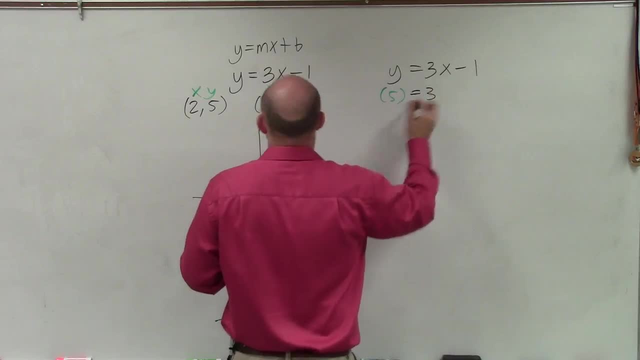 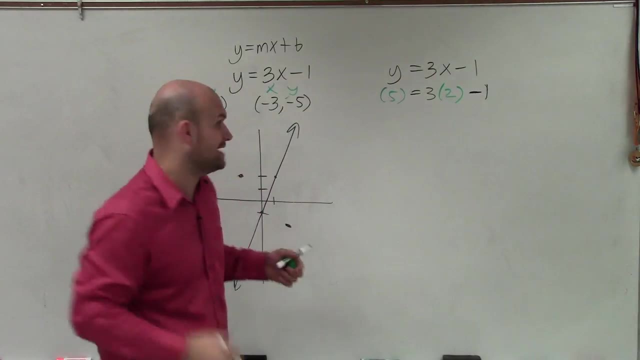 whole Airbnb. Now I need a slide, So I will plug in this cloth here here After gesagt for y and plug in a 2 in for x. Then I'm simply just going to evaluate and see if it's true or not. 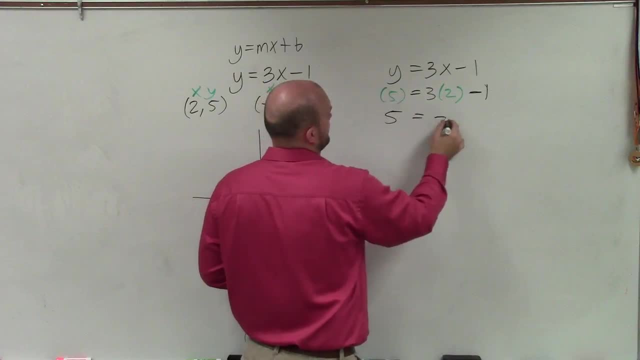 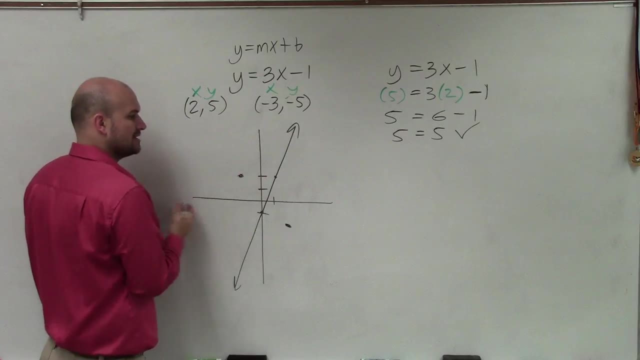 So 5 equals 3 times 2 is 6.. 5 equals 5.. That's true. So, since that's true, that means this point is on the line. So let's look at that graphly to make sure that's correct. 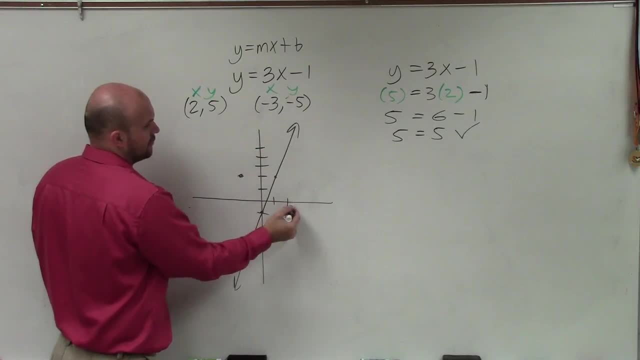 So I go over 2 and then up 5.. 1,, 2,, 3,, 4,, 5.. Over 2,, up 5.. I mean my graph's a little bit off, But yes, you can see it works. 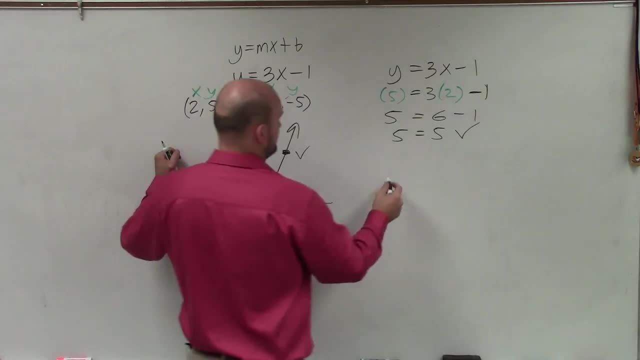 Now let's check the point: negative 3, negative 5.. So I have y equals 3x minus 1.. Now I'm going to plug in the points: negative 5 in for 3 and negative 5 in for y, I'm sorry- and negative 3 in for x. 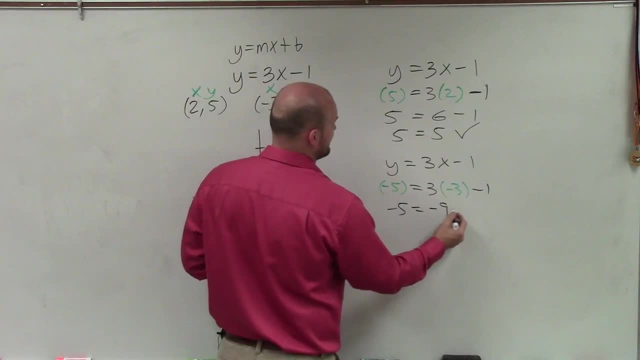 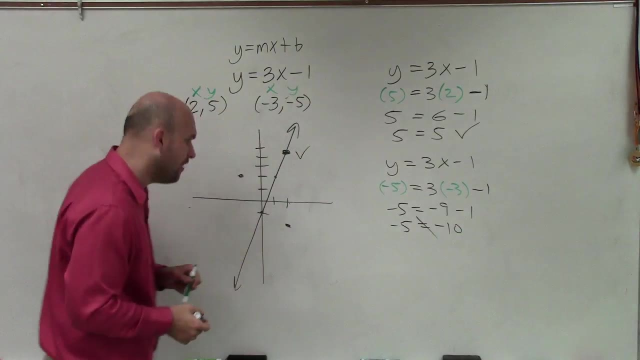 So negative 5 is equal to 3 times negative. 3 is negative 9 minus 1.. Negative 5 is equal to negative 10.. Well, negative 5 is never going to equal negative 10, so that is false. That means the point: negative 3, 5,, 1,, 2, 3, down 5, 1,, 2,, 3,.